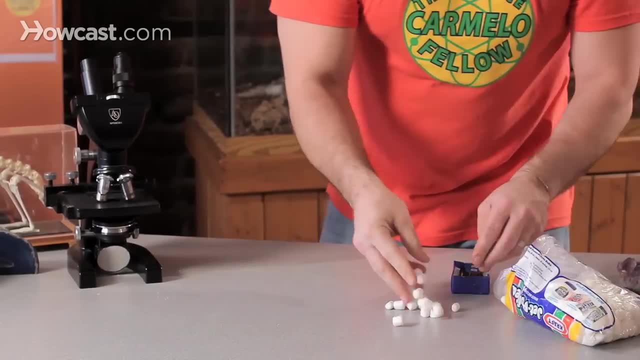 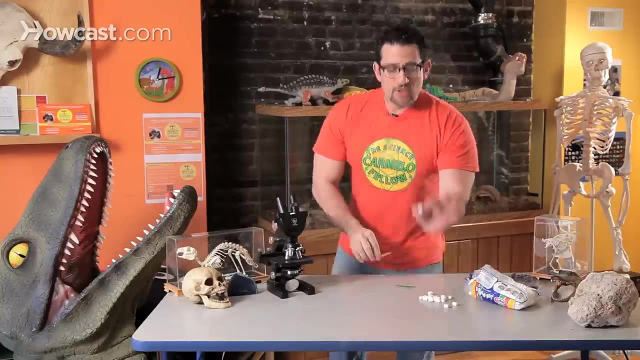 structure is actually going to be three-dimensional And all you need are marshmallows and all we need are toothpicks. It doesn't matter if they're the pointy type or the flat type, but marshmallows are actually cylinder shapes. 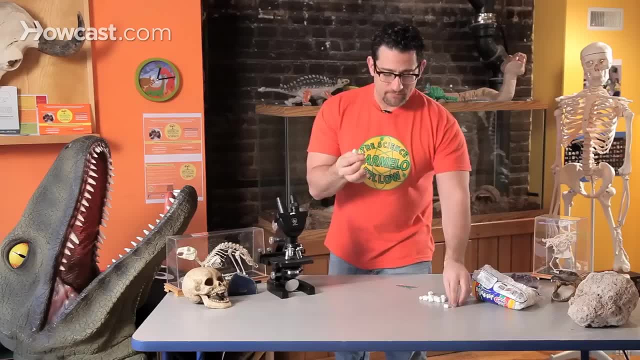 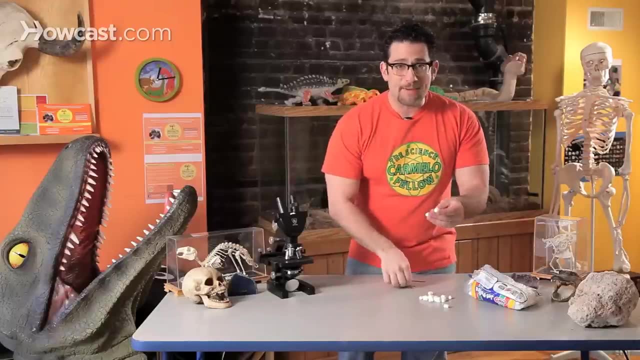 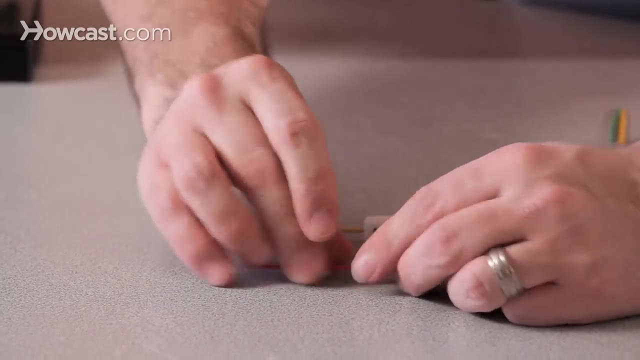 Okay, So take a marshmallow, take a toothpick, put it through. You kind of have it looks like you're going to be working out with it, right, But you're not. Now think about how we can take this and turn it into a really awesome three-dimensional shape. I'm going 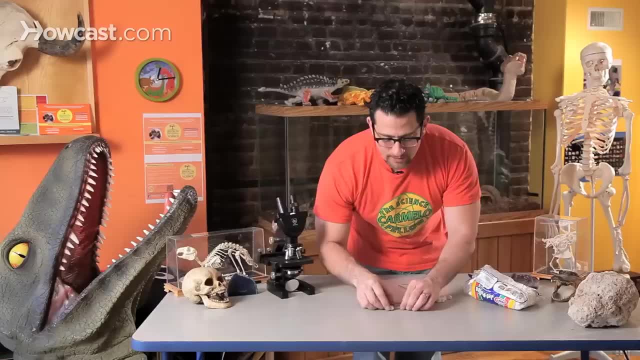 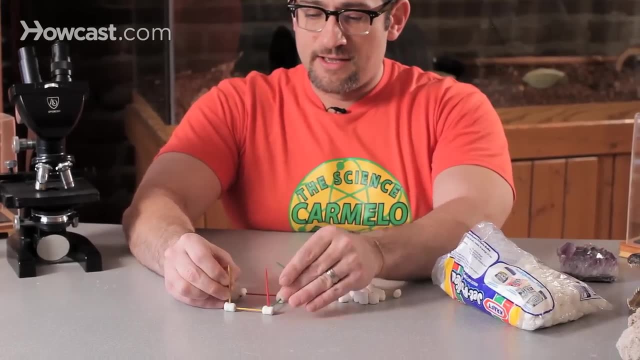 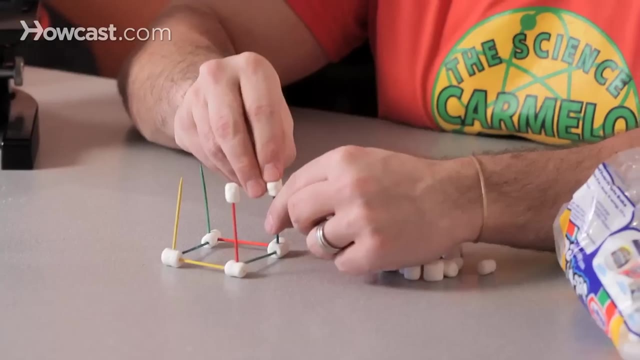 to start with a square, and then I'm going to build it up and turn this square into a cube. Now I'm going to start going higher, just like this, And the beauty about this experiment is a bag of marshmallows is so inexpensive. Toothpicks. 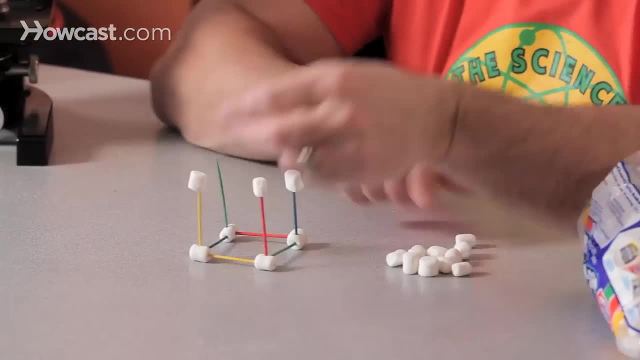 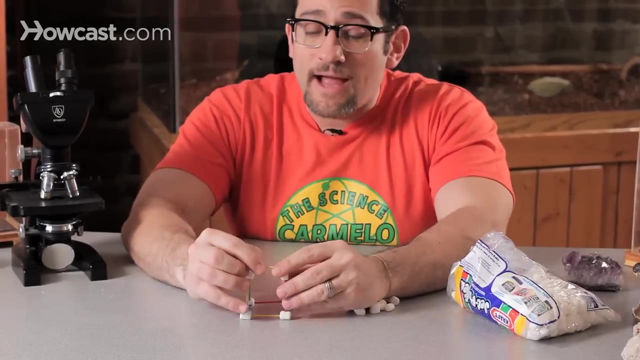 pretty much anybody has toothpicks at home And I could learn so many amazing concepts of engineering and building Gravity center of gravity. You see, you really want this structure, to have this amazing center of gravity, so that because, if you really think about 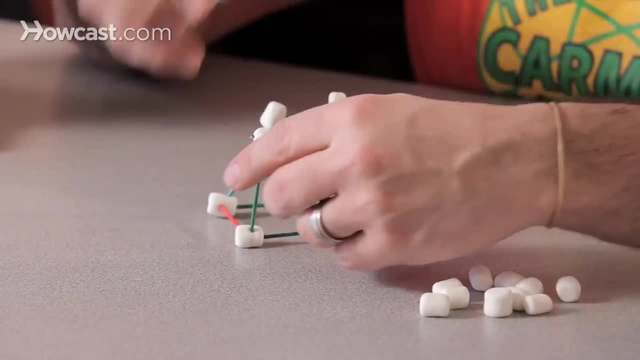 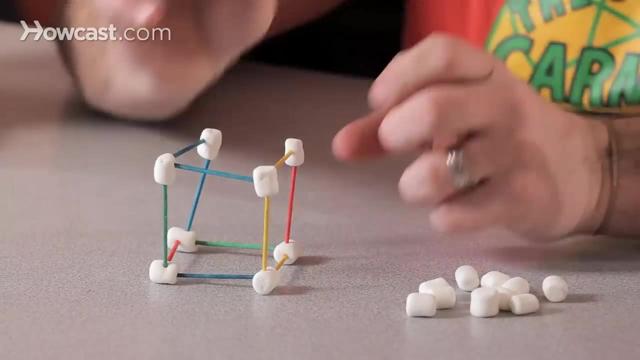 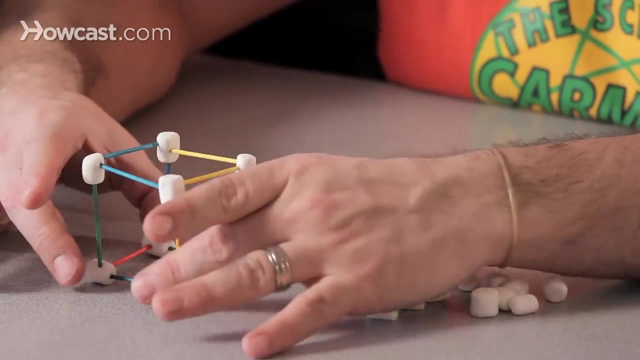 it. gravity's always trying to knock you down. Okay, In fact, unfortunately, when we get a little older, you start to lean. You start to lean forward because your lifetime, your body, has done nothing but battle gravity, which is why our backs arch as we get older. Okay, But now look, I just made a three-dimensional 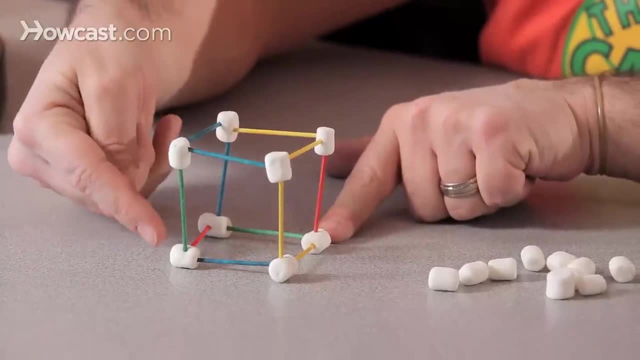 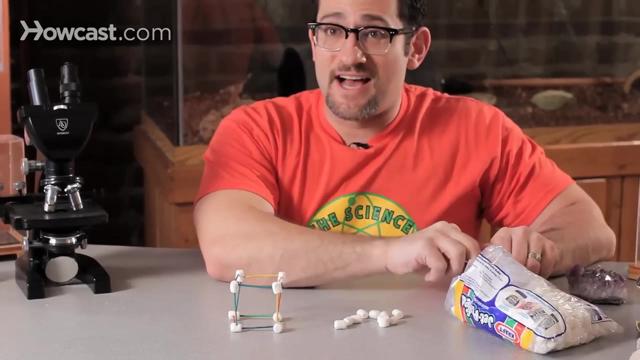 cube. This is exactly one floor high. But the challenge is, could you create multi-floors And as you get it to go higher and higher? okay, it has to be stable, stable on the table. You do not want it to be not balanced. 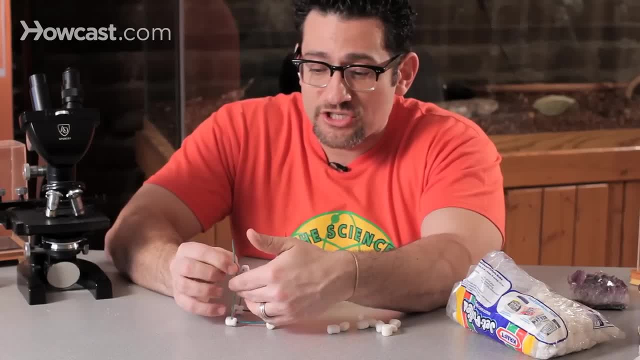 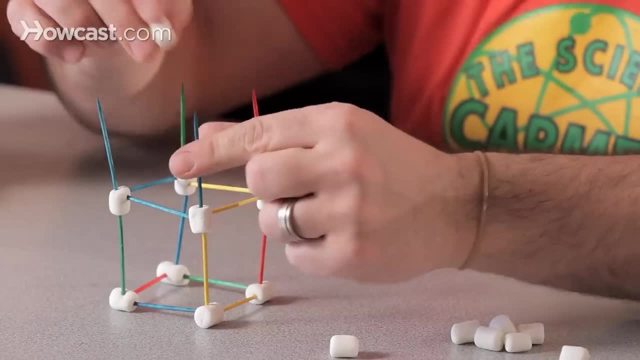 The rules are: you're not allowed to hold it up. This is a challenge. And you're only allowed to use toothpicks. You're not allowed to get scotch tape. Okay, That's the challenge, And, as you can see already, mine is starting to lean. Gravity's always pulling on it. I'm 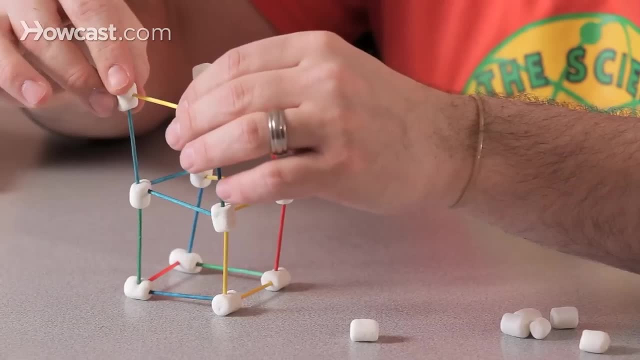 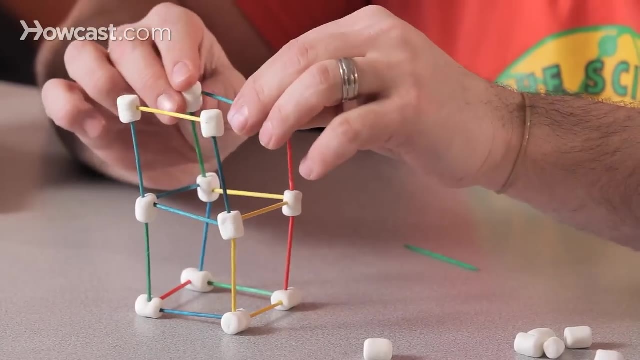 only going to make mine three toothpicks high, Just because I don't need to make it bigger. that's going to be your challenge. And then I'm going to simulate an earthquake, And then I'm going to see if my structure is still standing, And there are other things that